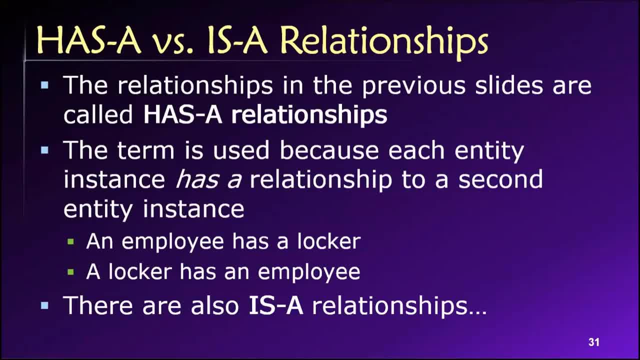 has relationships with is a relationships. Now, generally, most of the relationships that we've worked with thus far have been has a relationships. So we can say, for example, that, like an employee has a locker right, Or a locker has an employee, 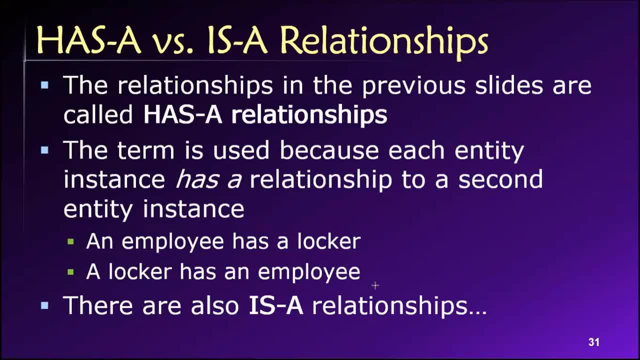 or a department has employees, an employee has departments right, An employee can have employee skills right. So these are all as a relationships, But there are also is a relationships that we'll get to here momentarily And this is a different, different sort of concept, but we need to learn how to. 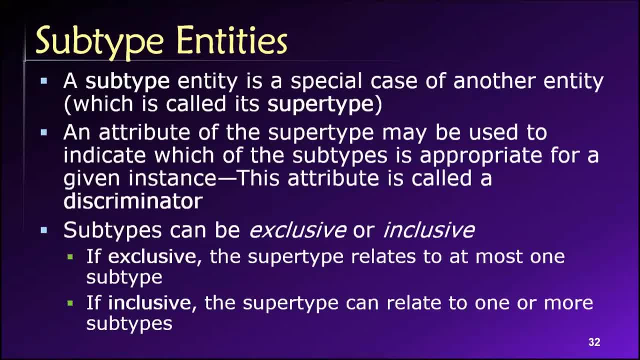 represent it in our entity relationship diagrams. So before we do that, let's talk about the difference between supertypes and subtypes. Now, these are very common in the real world, And hence it's good for us to have the skills to be able to model them, because we may 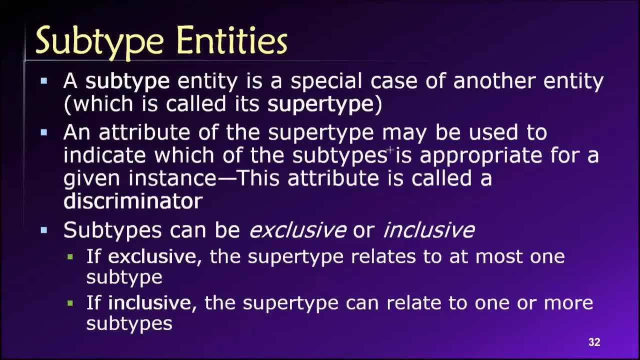 find ourselves in a situation where a company needs us to model a supertype- subtype relationship as part of our database design. So the basic idea here is one of inheritance. So a subtype is a special case of another entity which is called a supertype. 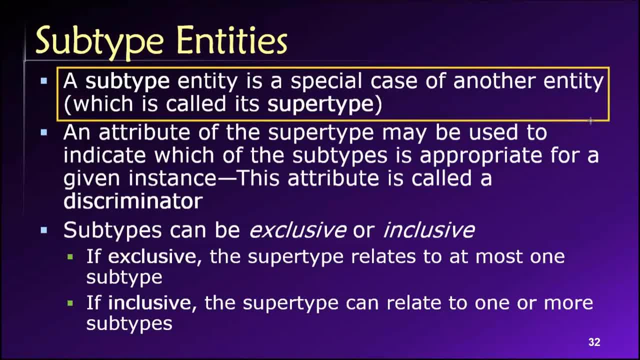 So here's an example. If you think about all of the people that are associated with a university, right, We're all people, but we play different roles. So we might say that maybe we take all the people associated with the university And one way to possibly divide them would be. 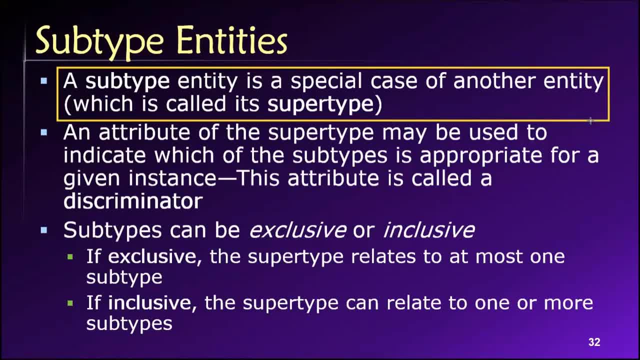 employees versus non-employees, So we might have a group of employees, We might have a group of students, right? Just like a company could say: like employees versus customers. Now, they're all people, They're all human beings, right, They're just special types of human beings One belongs to. 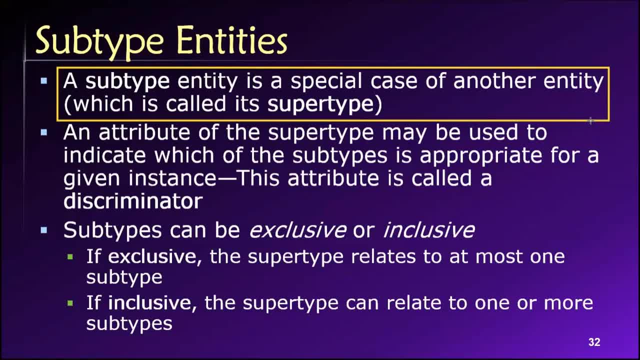 one group and the other belongs to some other group. At a university, a very common way of differentiating between the different special types of people that participate in the university community would be to label some of them faculty. Those are the people who teach right And then 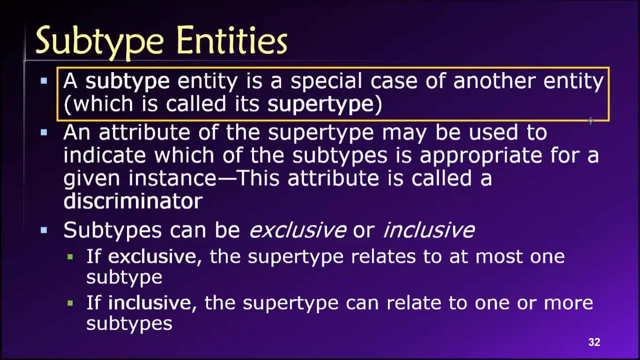 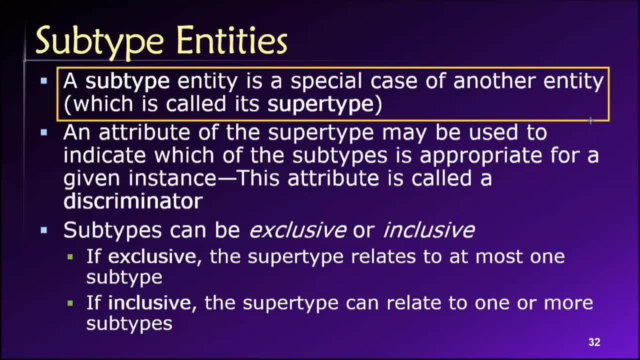 wanted to, we could divide the people at universities into three different subtypes. We could say the subtypes are students, faculty and staff And then, if we wanted to, maybe we further divide, say, students into undergraduate students versus graduate students. So we can. 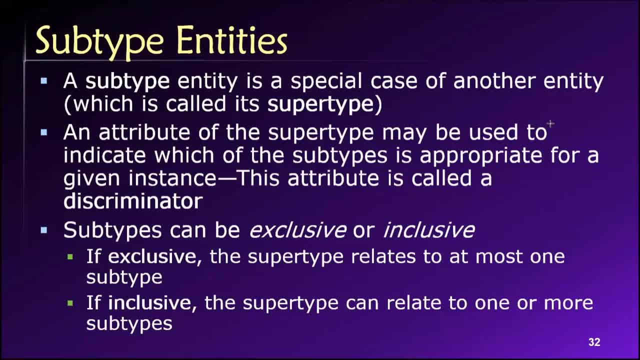 have subtypes of subtypes, But the idea here is that this is an inheritance relationship. Just because someone is a student doesn't mean that they are not also a person, right? It doesn't matter if you're a student or if you're not a student. It doesn't matter if you're a student or. 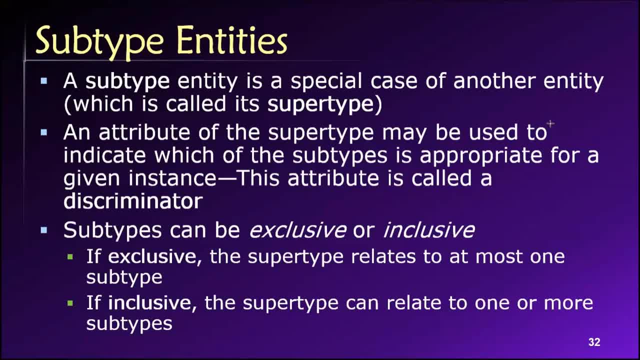 a staff member or a faculty member. you're all people, And this is what is known as an is a relationship, right, Because a student is a person, A faculty member is a person, A staff member is a person Or, in more of a corporate context, an employee is a person. 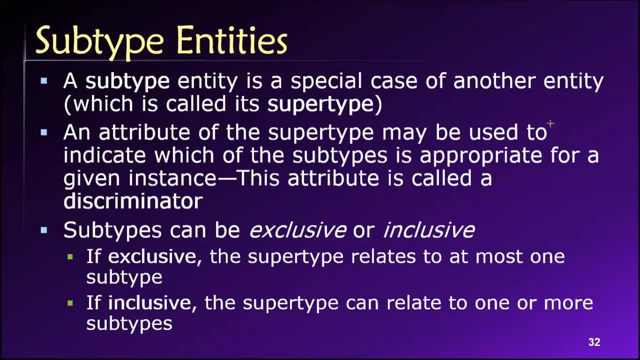 A customer is a person Or maybe some other entity like, maybe it's an organization, that's a customer right, But the notion here is is hopefully clear, And what we can do with these types of is a relationships is we can capture general information that is of interest to us. 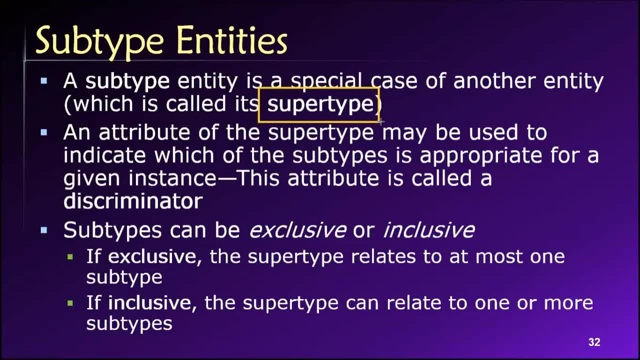 about the supertypes And then we can capture additional information about each subtype that is specific to each of those subtypes. So, for example, if I'm talking about people, regardless of whether you are a student or a faculty member or a staff member- 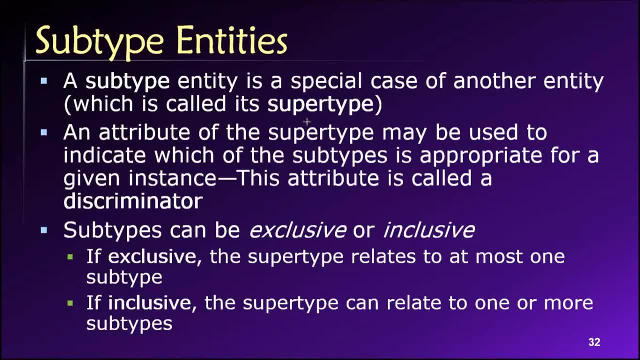 at the university. there are going to be some common things that I want to record about you in the database, like your campus-wide ID right. That applies to everybody, regardless of whether you're a faculty member, a staff member or a student. Your name right. Your mailing address. 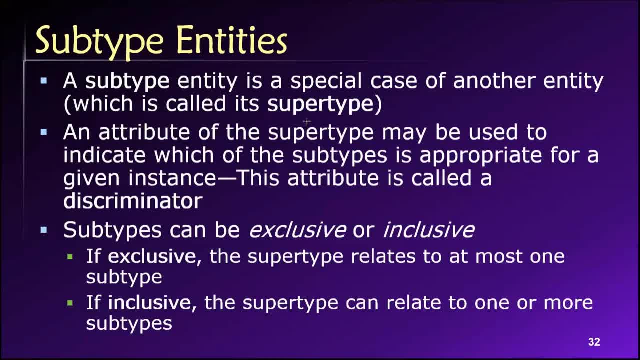 probably your email address, telephone, maybe your date of birth, right? So there, these are common attributes that we want to know about all people that are a part of our university community, regardless of whether they are faculty or staff or students, right? 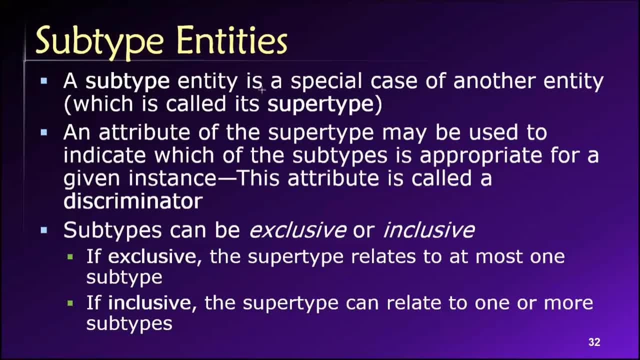 So this is our common set of factors, our common set of attributes, and we record those as attributes for the supertype. Now, and this is the key thing, is, depending upon which subtype a person might, we're going to record additional information about them that is specific to the. 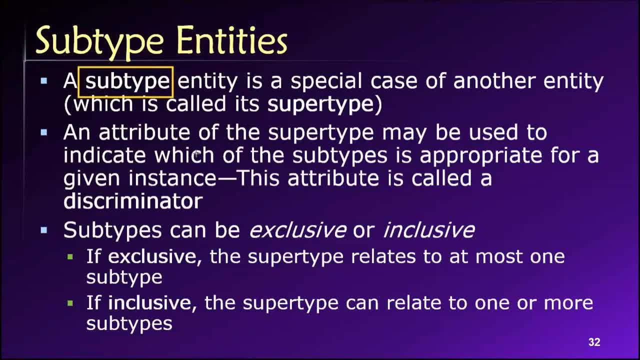 to that subtype. okay, So let's say, for example, that you are a student. Well, if you're a student, we're probably going to want to record information about your academic performance and your goals. So students are going to have things like a major or a concentration. They'll have grades. 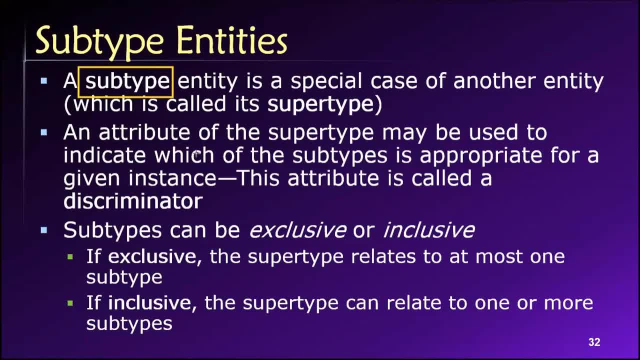 the courses that they've taken, the grades that they've earned in each of those courses, and so on, And these are things that are specific to the student role. right, If I'm a faculty member, I'm probably not going to have a major, or I'm not going to have grades or classes that I've 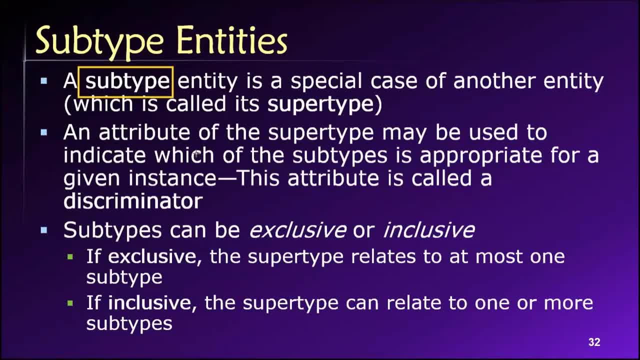 taken at this current university, So we're not recording that information about faculty. We'll probably record additional information about faculty that is not relevant to students: What is their office location? What is their office phone number? When were they hired? What is their salary? 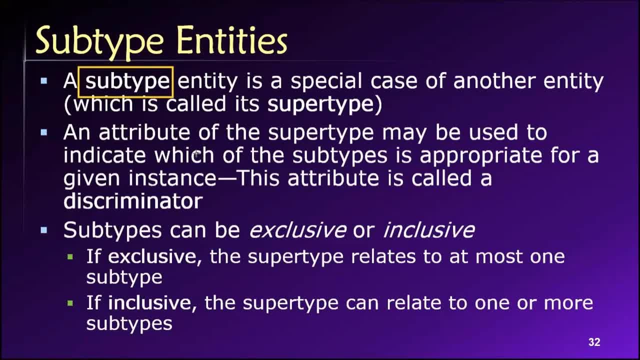 Like: these are all things that we want to record, like faculty members, that we would not want to record about students. okay, so, based on the specific subtype, we're going to record additional pieces of information, but we're going to have a common set of values or attributes that we record. 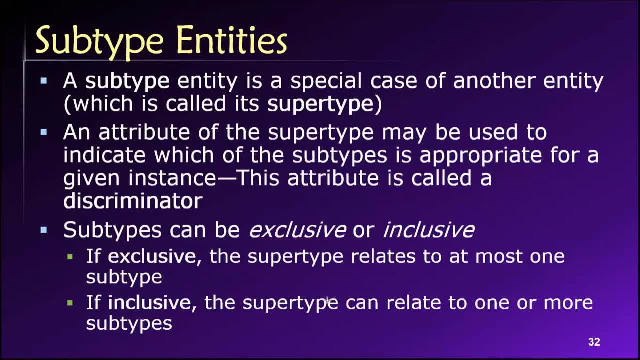 for our super types. okay, now, one additional thing- and then i'll show you some examples- is that these subtypes can be either exclusive or inclusive, and the difference here is simply: how many subtypes is a supertype allowed to be simultaneously? okay, so, for example, if i run my university in such a way that my staff members cannot be, 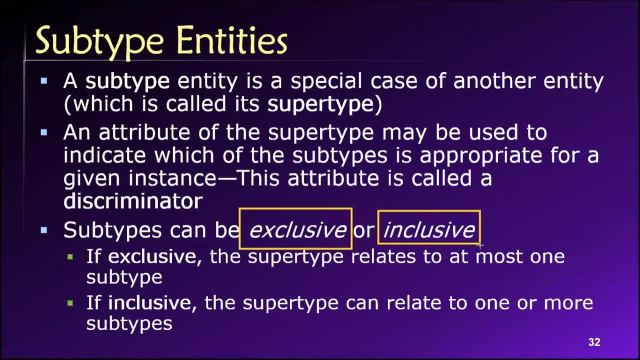 students as well. like you, must either be an employee of the university or a student. well, in that case it would be an exclusive supertype subtype relationship, because each person can only be one subtype at any given time. i cannot simultaneously be of two subtypes, but if it's possible, say, for example, for someone to be both a faculty member and 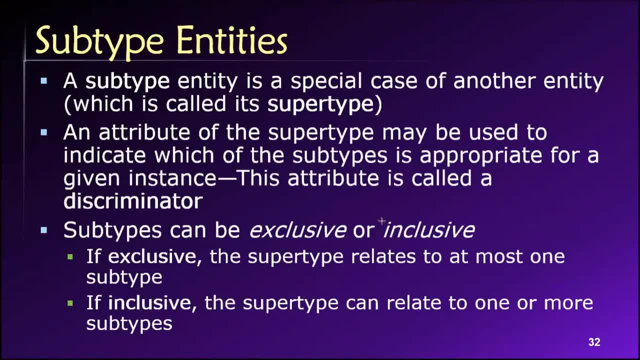 a student simultaneously at the university, then it's going to be an inclusive supertype- subtype relationship because it means that that person- remember, in this example the person- is the supertype. it's the generic concept that person could simultaneously be playing two roles at the university. they could be a student and a faculty member and that means they could. 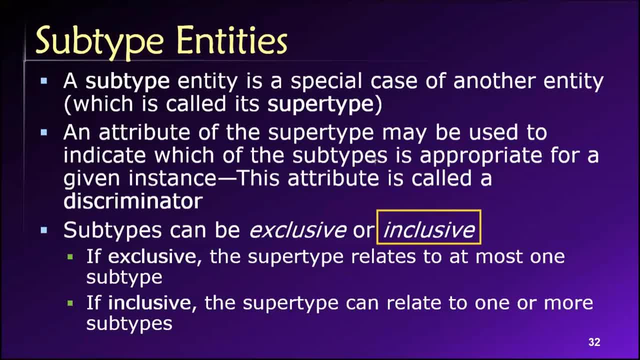 simultaneously be members of two different subtypes, or maybe even more. okay, so this is an inclusive supertype- subtype relationship. all right, so i've talked about this in text form. let's see some examples as well. okay, so here are some of the models that we're going to use on our course. 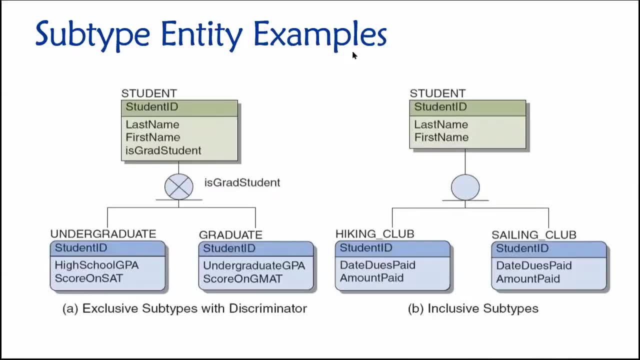 examples. This is easiest to understand with some lovely pictures here. All right, So what we have here, then, are two supertypes which you will notice are strong entities, And so this is a student supertype here and a student supertype here, And we're going to model two different. 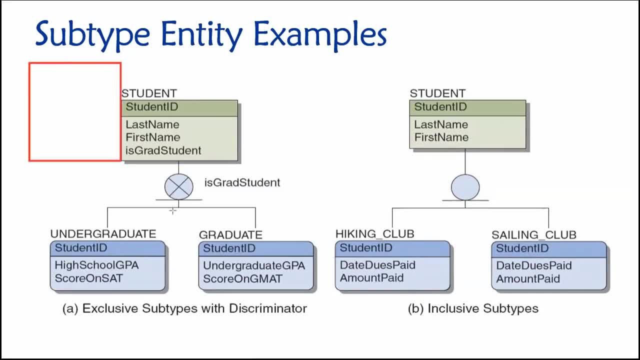 relationships. The first one, which is shown over here on the left, is an exclusive supertype, subtype relationship, And we can see that in all of these that we have this sort of circle symbol right That then branches off into the various subtypes, but this circle symbol has an X in it. 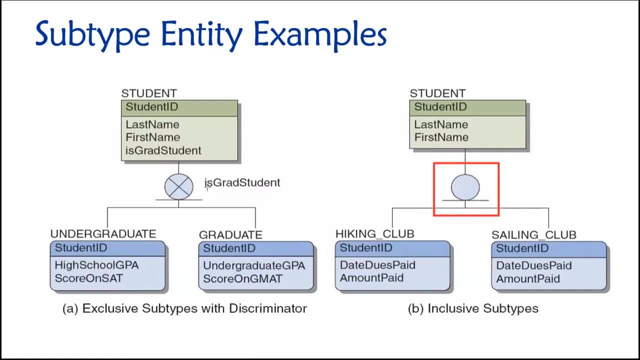 And if you contrast that with the one over here, you'll see this one does not have an X. So the way that I remember this- and hopefully it works for you- is X is exclusive. I know it doesn't really work out from a spelling perspective, but you can think of it that way. 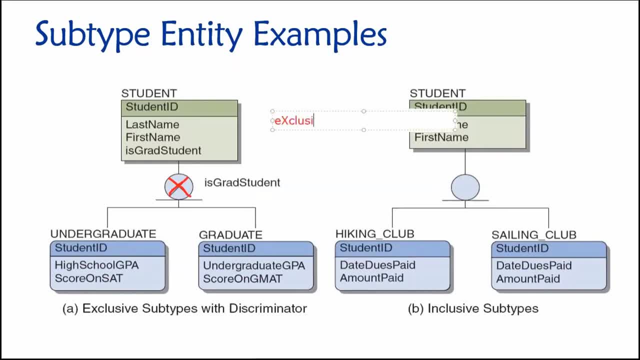 I don't know, maybe like this, like exclusive right, I said the big X, So that is our visual symbol: that this is an exclusive supertype, subtype relationship, meaning that each person, in this case each student, can only be one of the subtypes at any moment in time. Okay, So in this case, 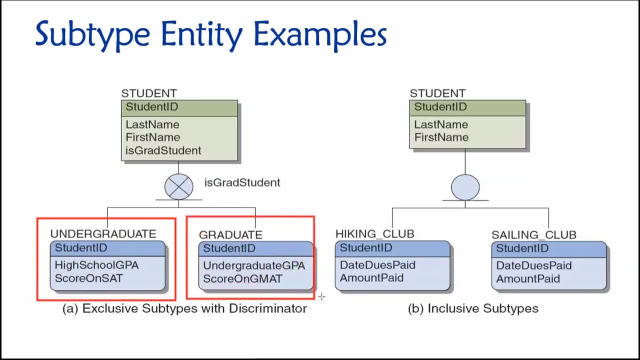 our subtypes are undergraduate versus graduate, And it makes sense in a university scenario to say that a student must be either an undergraduate student or a graduate student, right, We cannot allow the same student to simultaneously be in both of those roles. So what this means from a data perspective is we're going to have this undergraduate table. 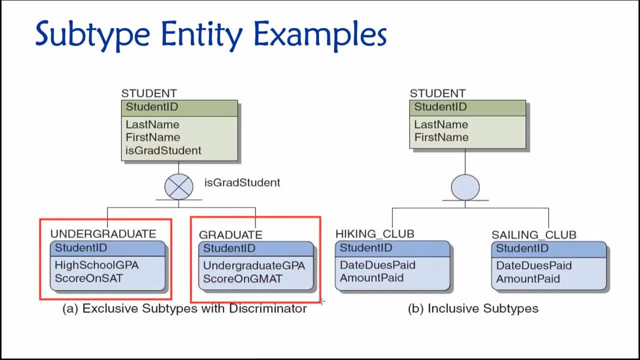 down here. right, This is a subtype table and we're going to have this graduate table And you can see that we use the student ID, which is the primary key from the parent table, as the identifier. So in each of these cases, the student ID is serving. 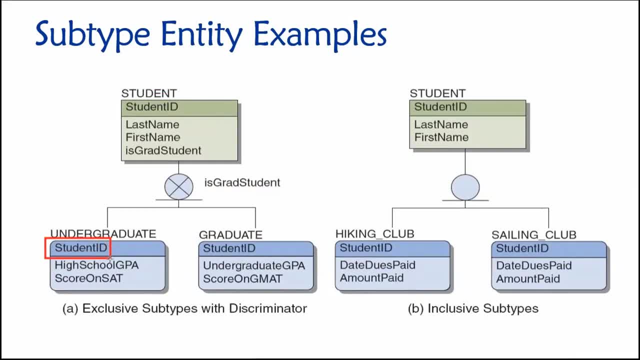 both as the primary key of the subtype table and also as a foreign key link back to its parent table. However, because this is an exclusive supertype subtype relationship, we need to know to which subtype does each student belong, And that is determined using this attribute right here. So we've created this attribute. 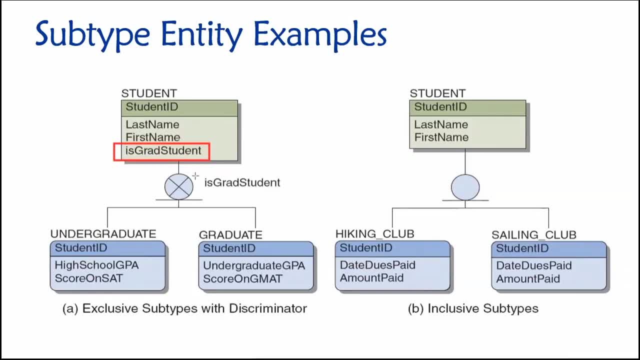 you can see, it's a simple Boolean or bit attribute which is going to hold like a true or false, yes or no, one or zero, indicating whether a particular student in the student table is a graduate student or not. So if the value of that attribute is true, then we're gonna follow this path. 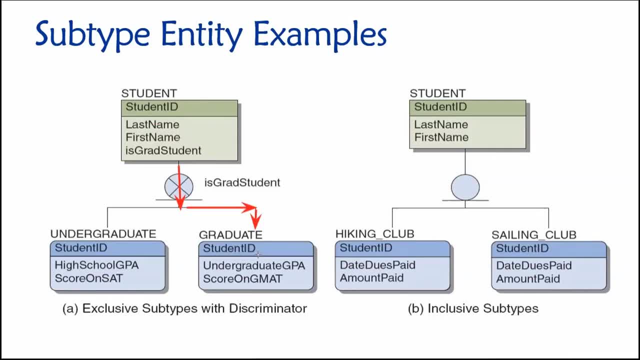 And we can get additional information about that student by looking in the graduate student table. right, If the value of is grad student is false, then we would follow this path and we would get additional information about that student by looking in the undergraduate table. 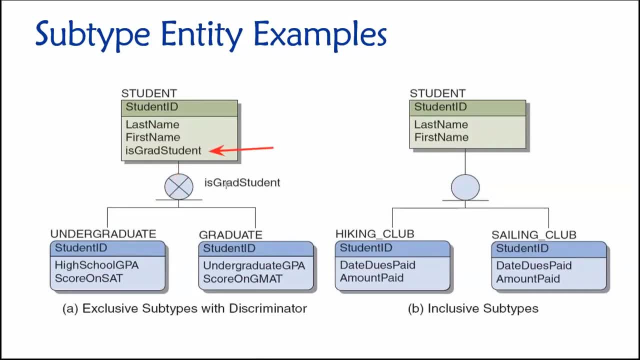 So this attribute is called a subtype discriminator, because it tells us which of these paths we should follow, And this only applies and is only used in scenarios where it is an exclusive supertype-subtype relationship, because we're only going to follow a single path to just one subtype. 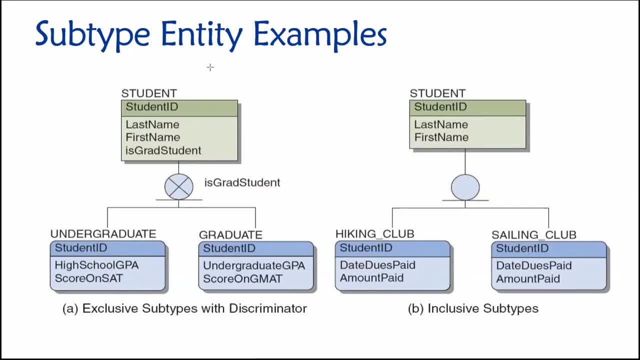 Now remember, the idea here is: it's just like inheritance. So if you studied object-oriented probe with this idea of inheritance, right, you can have an abstract class, in this case an abstract concept, like a student, And then you're going to have specific types. 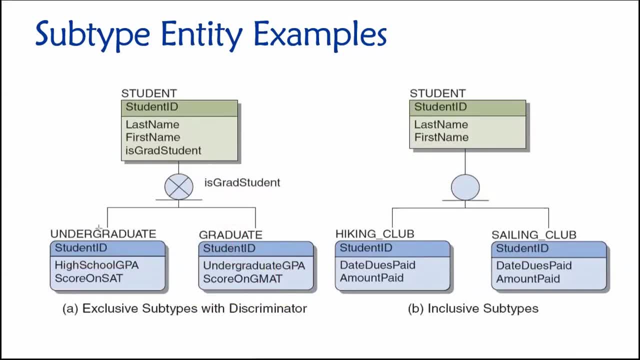 Types of students, like undergraduate versus graduate. But the point here is to note that an undergraduate student is a student. A graduate student is a student. So if I'm looking at I don't know, maybe student number seven and let's say that that student is a graduate student. 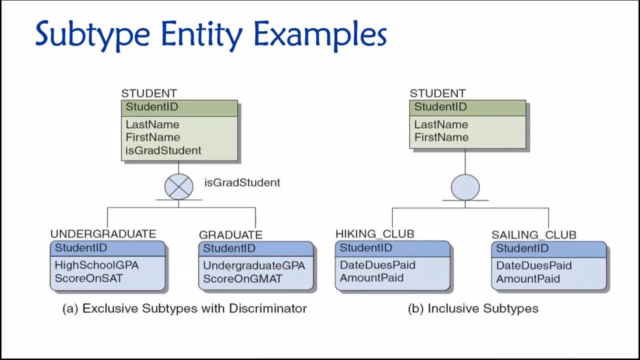 And I said what attributes are associated with student number seven. The answer is student ID, Last name, first name and whether they're a graduate student, as well as these additional attributes down here which are only of interest to us as a university, if a student is a graduate student, right? 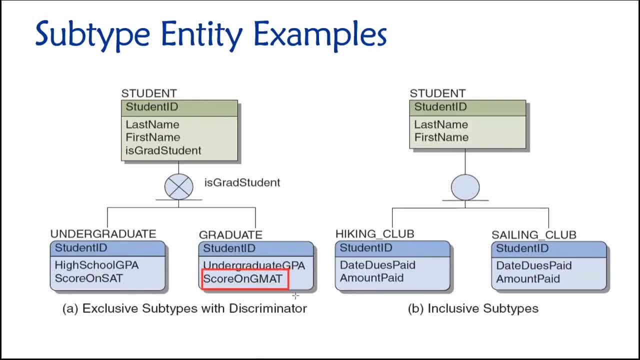 Like, graduate students in business commonly take the GMAT right. So if somebody is not a graduate student but instead is an undergraduate student, I probably don't need to record their score on the GMAT Because they're not a graduate student yet. 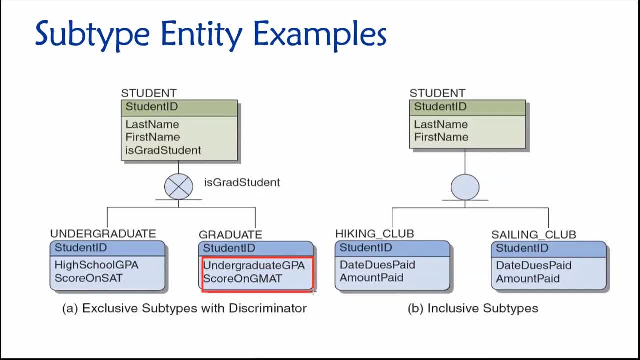 A graduate student is a student. If I ask you something like you know what attributes are associated with graduate students. it's all of these right, Because our specific type of student- graduate student- inherits all of the attributes of this supertype as well, right? 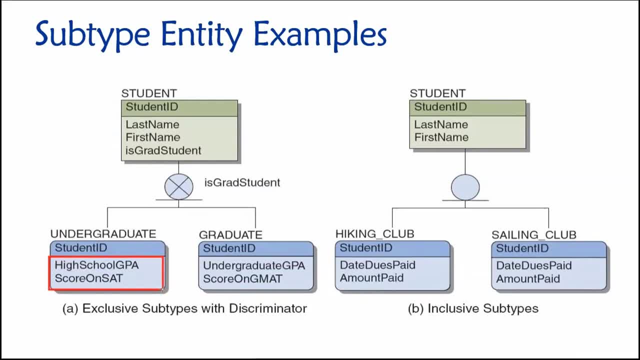 Same with undergraduate. Here we have a set of specific attributes that apply only to undergraduate students, But we have this common set of attributes that applies to all students. So if I said you know what are an undergraduate student's attributes, It's student ID, last name, first name, whether or not they're a graduate student, and their high school GPA and their score on the SAT, which you know is an entrance exam for admission to the university as an undergraduate. 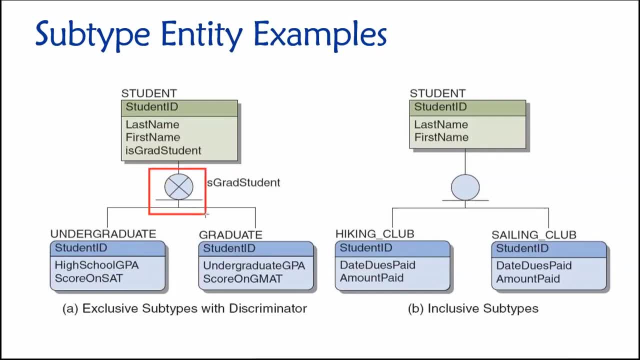 Okay, So that is an exclusive relationship On this side. over here on the right, we have a set of attributes. On this side over here on the right, we have an inclusive supertype-subtype relationship. So we still have our student table up here with student ID, first name and last name. 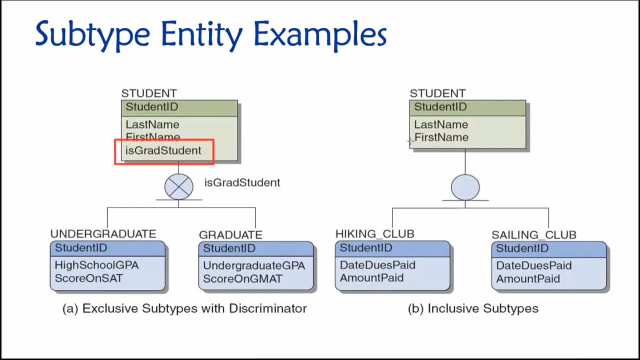 Note that there is no subtype discriminator attribute. Okay, So this is not used in the case of inclusive relationships. We do not have an X inside this circle, So it's not exclusive. Okay, That's how you could remember that X for exclusive. 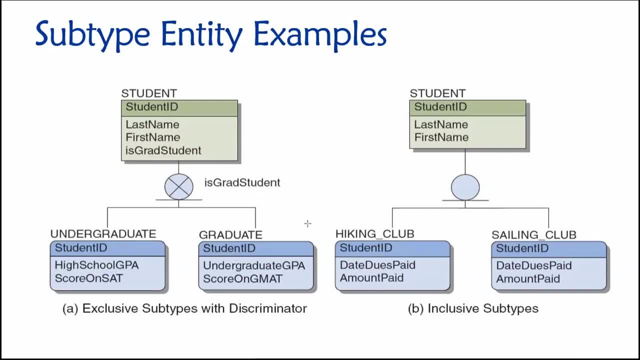 This is an inclusive supertype-subtype relationship. In this case the subtypes are tables about clubs And you'll note again, we use a single identifier, a single key: student ID, which is the primary key of the supertype. 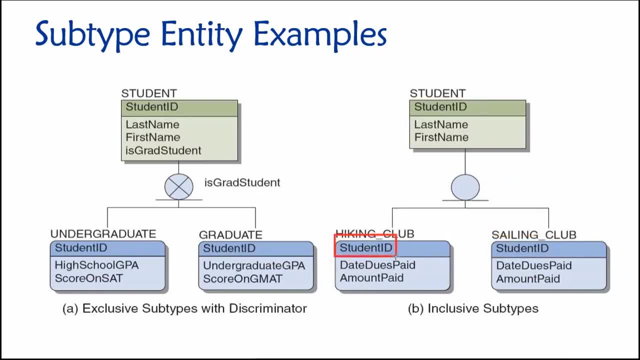 Down here in the subtypes. it serves both as a primary key and a foreign key. Back to the supertype, the student supertype. But the idea here is this is an inclusive subtype, So each student potentially could be added to one or both of these tables. 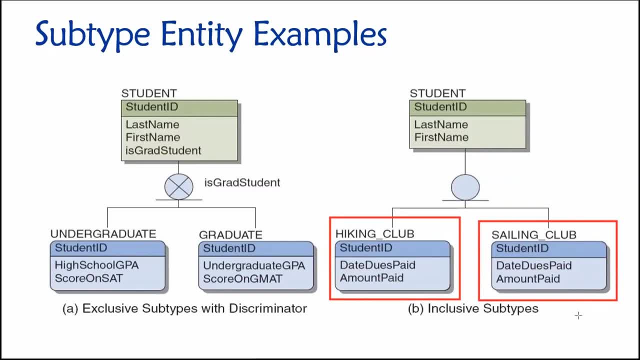 So if I'm a student, I can simultaneously be a member of the hiking club and the sailing club. Right, I don't have to choose one or the other. Okay, I don't have to be an undergraduate or a graduate student. It's like you could be both simultaneously. 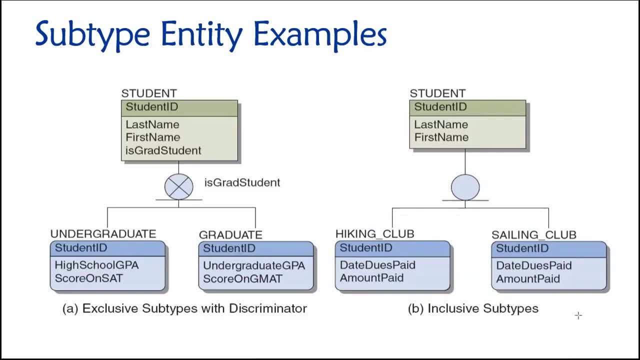 In this case I can simultaneously be a member of multiple student clubs. So this is an inclusive supertype-subtype relationship. So again, the difference is just: am I allowed- whatever the supertype is is an instance of that allowed to participate in more than one subtype simultaneously? 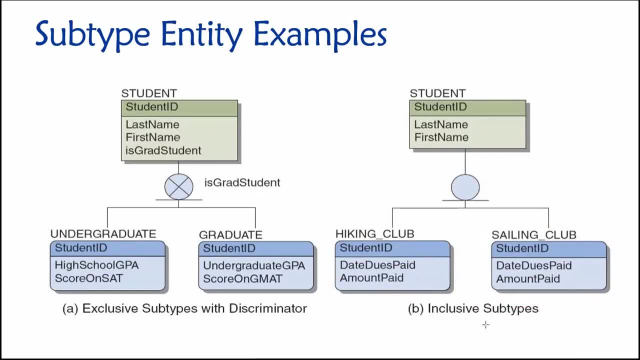 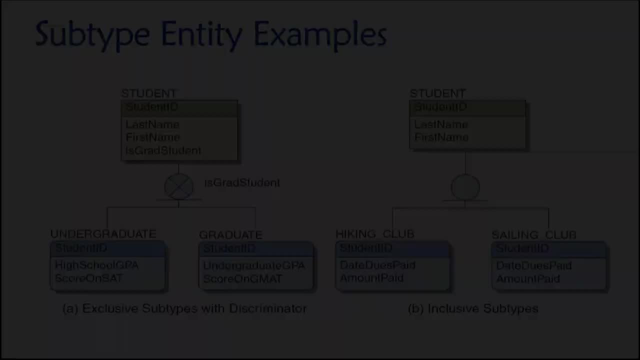 Like we see here, If the answer is yes, it's an inclusive. If the answer is no, we see over here- it is exclusive. meaning that each instance of the supertype student must be only one of the subtypes at any moment in time.